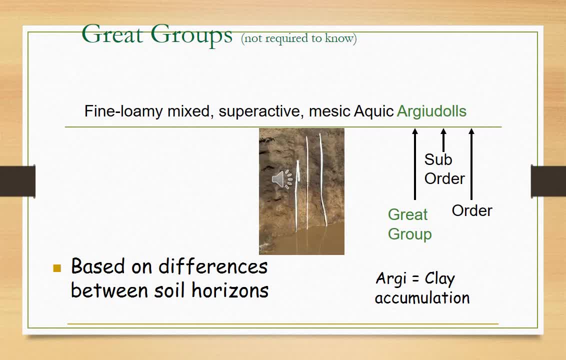 They have been established largely on the basis of differentiating soil horizons and soil features. Diagnostic Horizons: Soils in a given grade group have the same kind and origin as others. arrangement of these horizons: more than 240 grade groups have been identified. 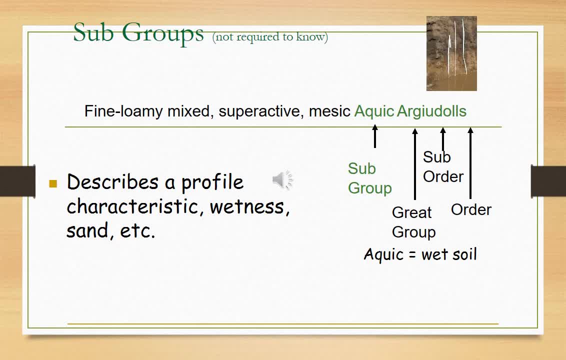 each soil grade group is divided into three kinds of subgroups: one representing the central concept of the soil groups, a second which has properties that tend towards other odors, subodors or other grade groups. and a third which has properties other than those listed in first two categories. 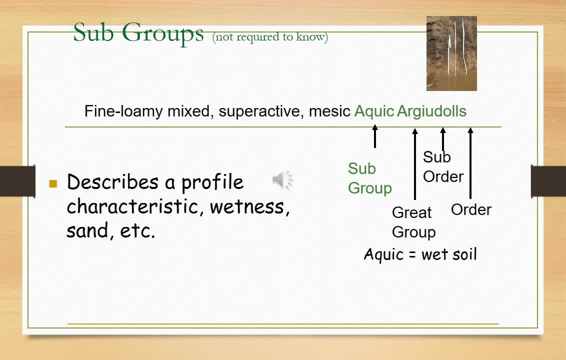 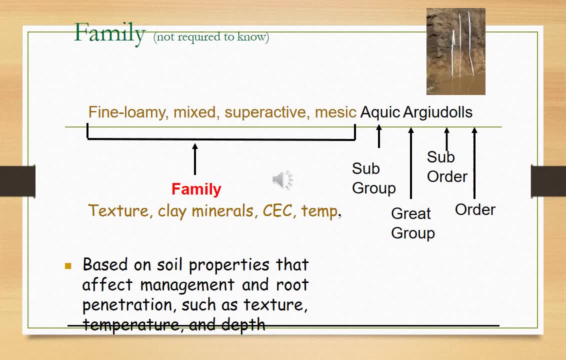 more than 1,200 subgroups are recognized. soil families are separated within a subgroup primarily on the basis of soil properties important to the growth of plants. some of these soil properties are texture, mineralogy, pH and distribution of rainfall and structure, as you can see here. 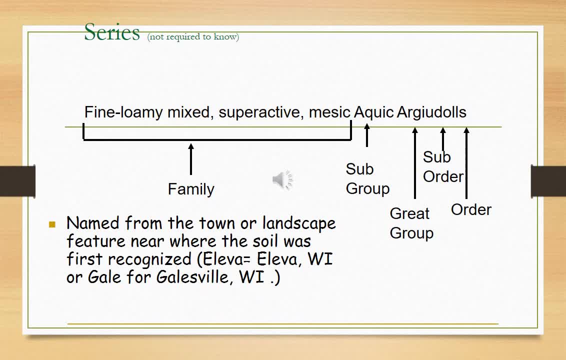 in this slide. as shown in this slide, the name of series has no pedogenic significance. it represents a prominent geographic name of a river town or an area where the series was first recognized. soils in the same series have similar properties, such as color, texture, structure, consistency, thickness, pH number. 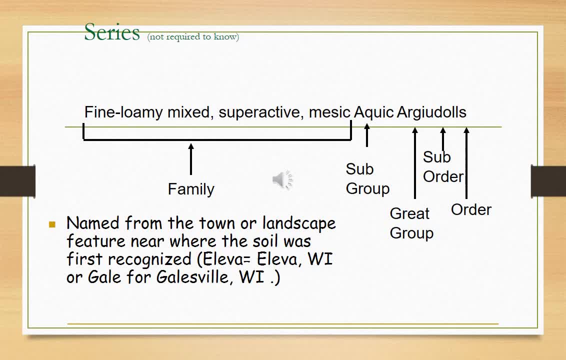 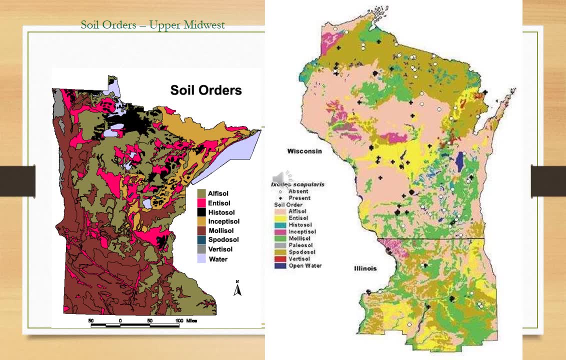 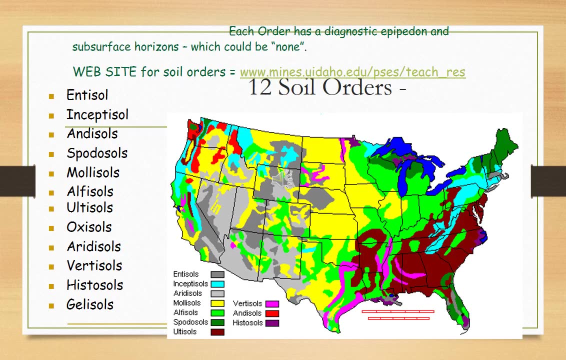 and arrangement of horizons and their chemical and mineralogical properties. different color show the different odors and subodors in the soil taxonomy. as you can see here in this slide, each odor has a diagnostic epipedon and subsurface horizons, which could be none. there are. 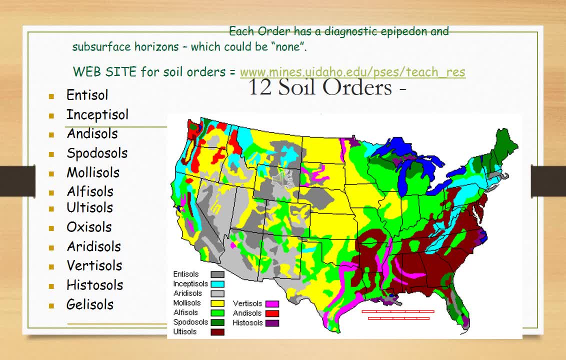 12 soil odors, that is, antisol, enceptisol and antisols: spodosol, molisols, alfisols, altisols, oxisols, eridisols, vertisols, histosols, xylisols. the different color shows different soil. 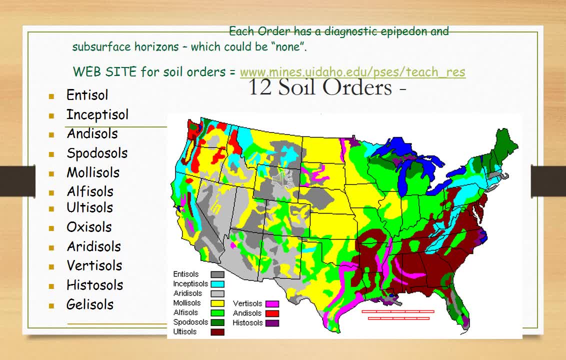 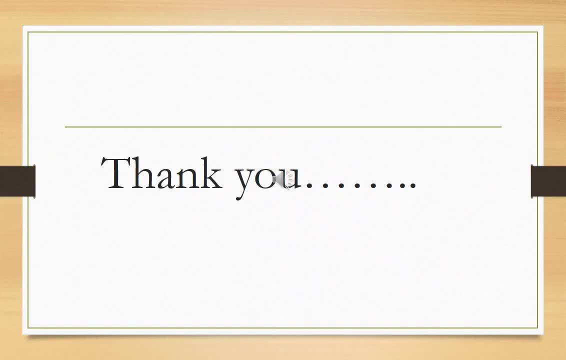 odors, which will be discussing tomorrow in the next session. thank you, stay home, stay safe.